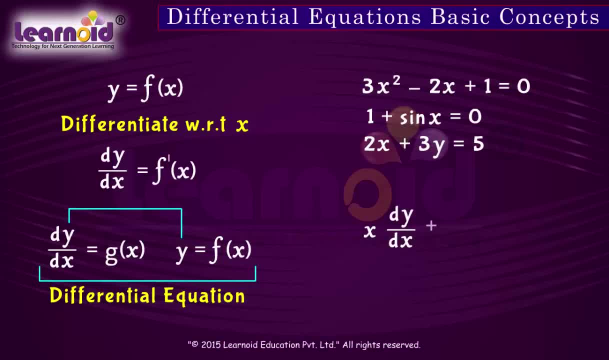 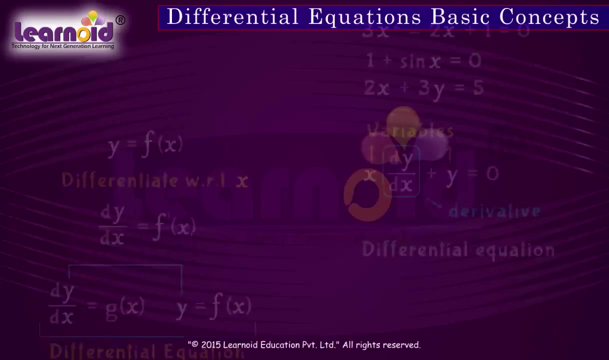 the equation x, dy by dx plus y is equal to 0.. This equation involves variables x and y, as well as derivative of dependent variable y with respect to x. Such equation is called as a differential equation, A differential equation involving derivatives of the dependent variable with. 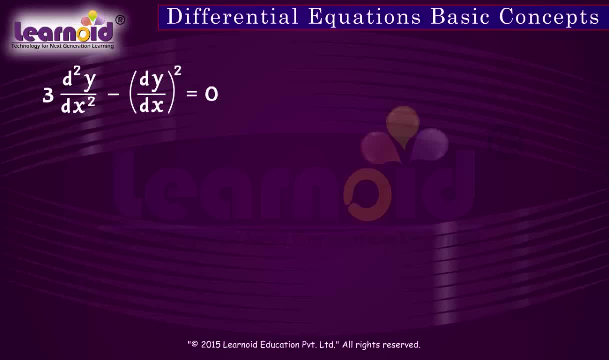 respect to x, respect to only one independent variable, is called an ordinary differential equation. While writing differential equations, we may be using notation y' for dy by dx, y'' for double derivative and y'' for triple derivative. Before finding methods to solve a differential equation, we will discuss order and degree. 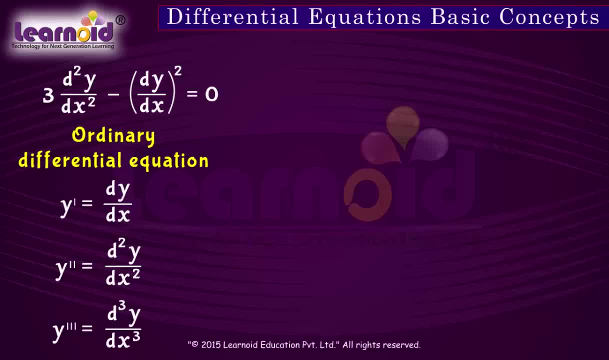 of differential equation. Order of a differential equation is defined as the order of highest derivative. in the given differential equation, Order of dy by dx is 1.. d square y by dx square is 2.. And d cube y by dx cube is equal to 3, and so on. 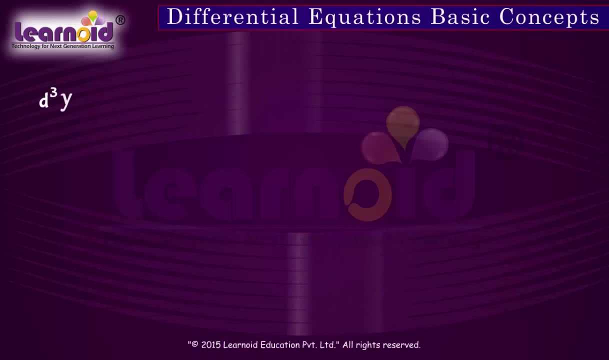 Order of differential equation d cube, y by dx cube minus x cube into d square y by dx square cube is equal to 0.. And its order is 3.. When the differential equation is a polynomial equation of derivative Y' Y'', Y''. 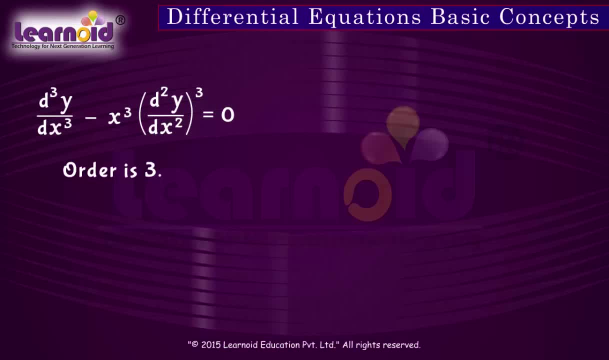 Y'' etc. We will find degree of the differential equation. The degree of a differential equation is the highest part of the highest order derivative in the given differential equation. Higher order derivatives can be written as y with super suffix, For example nth root 2.. 2., 2., 2. d, 3. 1, 2. 2., 3., 4., 1. And 2. 4., 2., 5., 5., 6., 6..